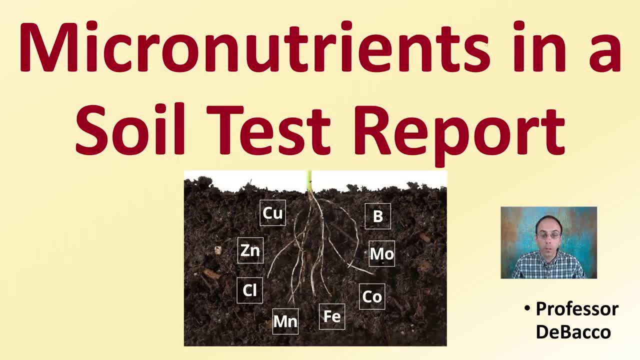 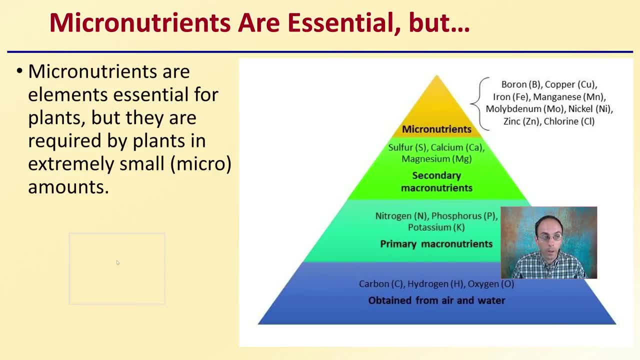 All right, let's look at micronutrients in a soil test report And here we see just a couple of them listed here in the image here. So let's look. micronutrients are essential, but so micronutrients are elements that are essential for plants, but they are required by plants in. 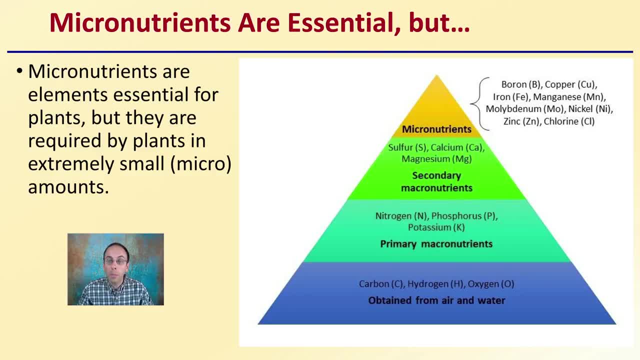 extremely small micro amounts. So when we're keeping in mind these micronutrients, we see a couple. here I see a little triangle. These are these kind of micronutrients: boron, copper, iron, manganese, molybdenum, nickel, zinc, chlorine- all considered to be micronutrients needed. 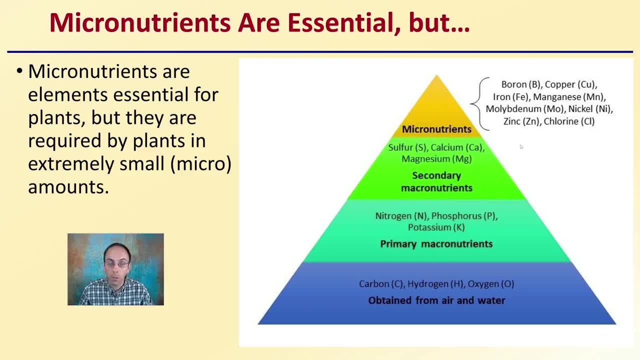 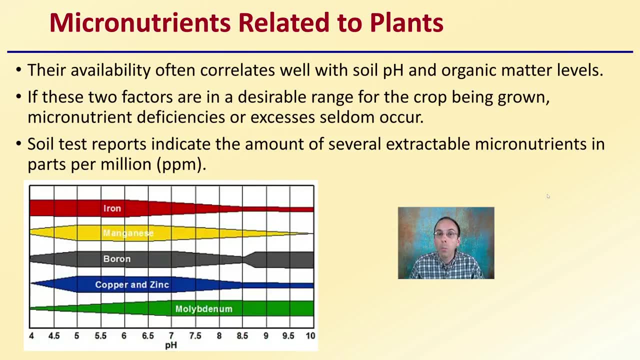 essential by a plant, but needed in very small micro amounts. So when we're looking at micronutrients related to plants, their availability often correlates well with soil pH as well as organic matter levels. So if these two factors are in the desirable range for the crop being grown- micronutrient deficiencies or excess. 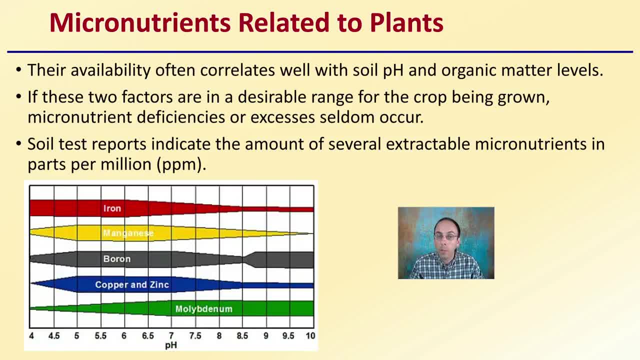 seldom occur. Soil test reports indicate the amount of several extractable micronutrients in parts per million, And this is again where you see that pH being a very important driving factor, Particularly for your micronutrients, because they're needed in small amounts, making sure your 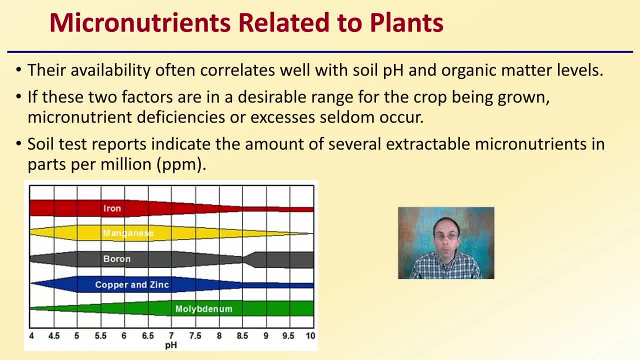 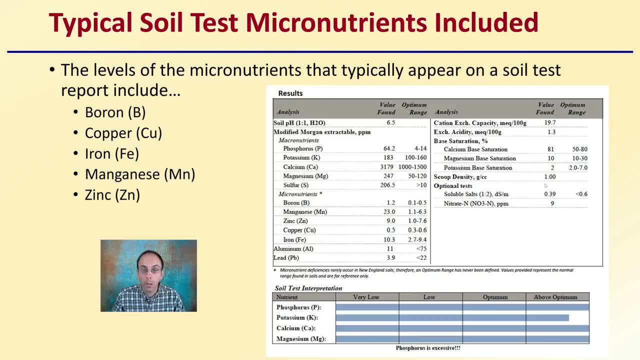 pH is dialed in can really help forego the potential for a lot of issues with micronutrient deficiencies. Now, typical soil test does include micronutrients. We can see one here provides boron, copper, iron, manganese and zinc. So the levels of micronutrients that typically appear in 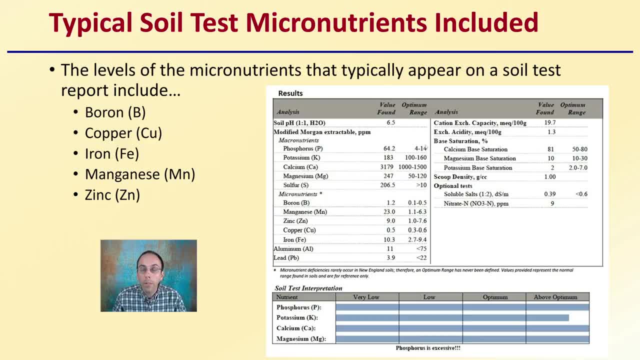 a soil test and we can see them listed right here. Then they give the kind of optimum range here Now a little different for the micronutrients compared to the macronutrients And as stated here on the micronutrients, you see this little. 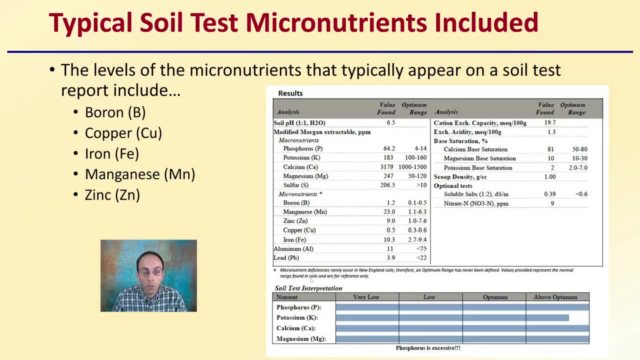 asterisk And in this soil test report it says micronutrient deficiencies rarely occur in New England soils. Therefore an optimum range has never been defined. Values provided represent the normal range in soils that are for reference only. So that's an important note For your. 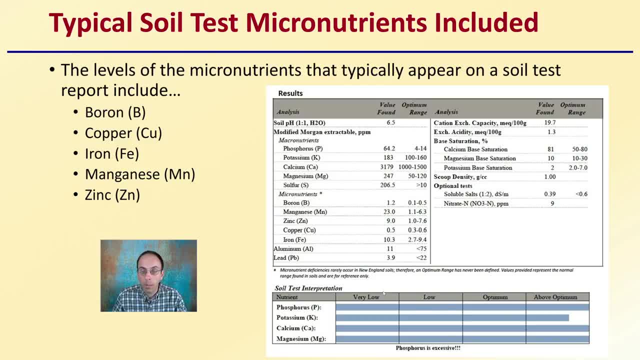 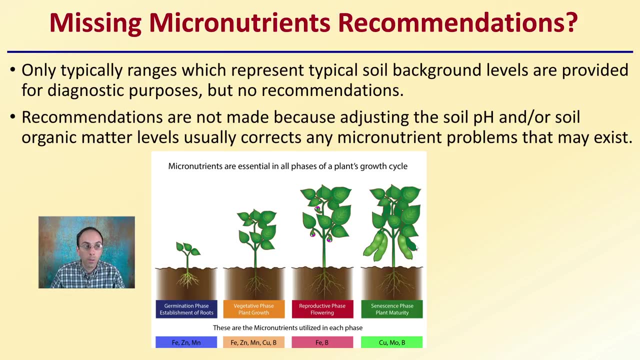 macronutrients we have an idea of an optimum range. That's why we see this very low, low optimum and above optimum range. But for micronutrients we're just providing with that general expected range for the region that the lab is from. So, as I said, missing micronutrient recommendations. yes, that's true, Only typical.